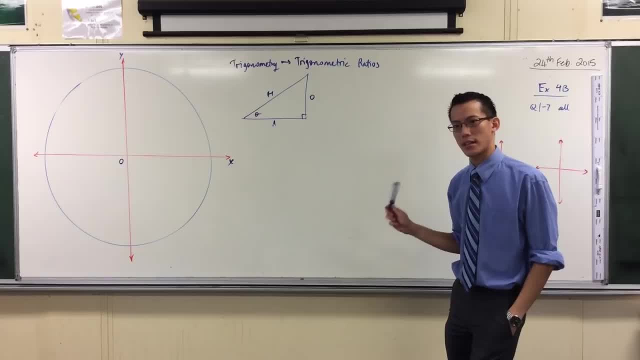 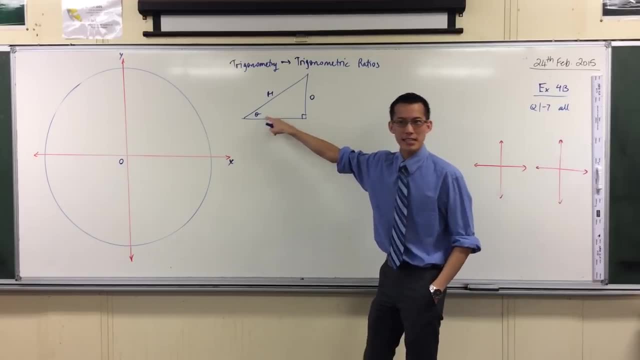 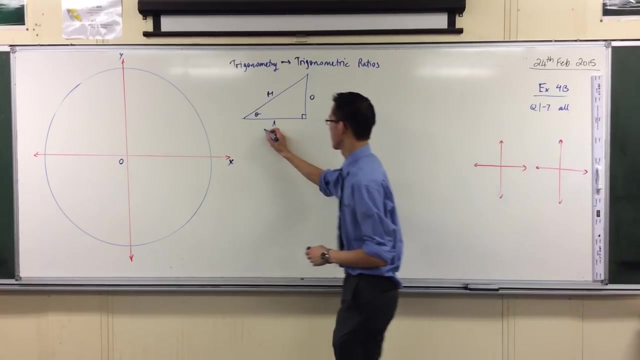 different ratios. but theta- and we notice this in our proof by contradiction about the tangent being perpendicular to the radius, we notice that theta automatically is locked into a certain domain. There are restrictions on theta. What are the restrictions? The 0, in between 0 and. 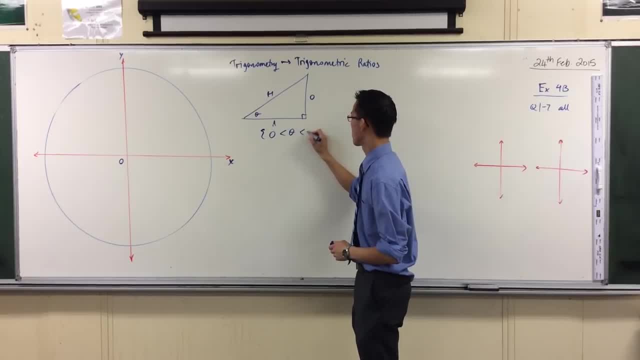 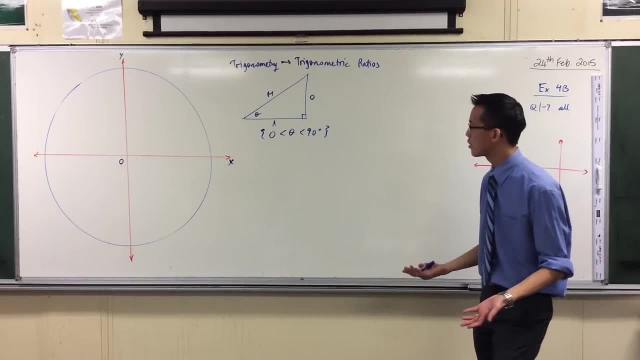 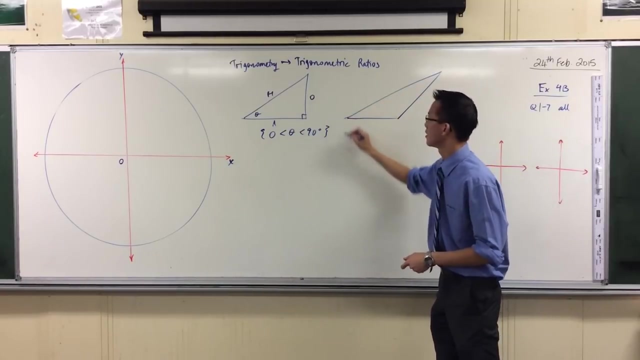 Good. so yeah, theta's acute. basically, right, This is, this is a problem, because if we want to understand angles, right, We don't even have to leave triangles. If I just push this triangle over to the side, right, Like, so okay, Like there's an angle. 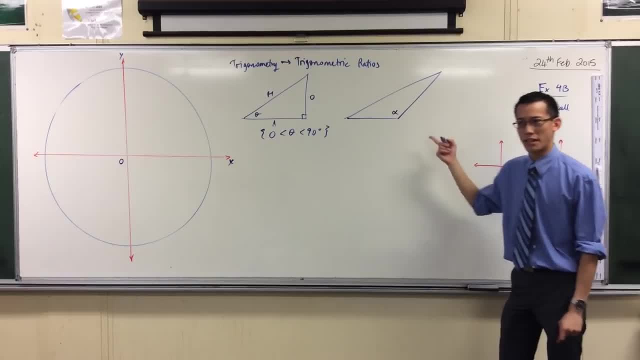 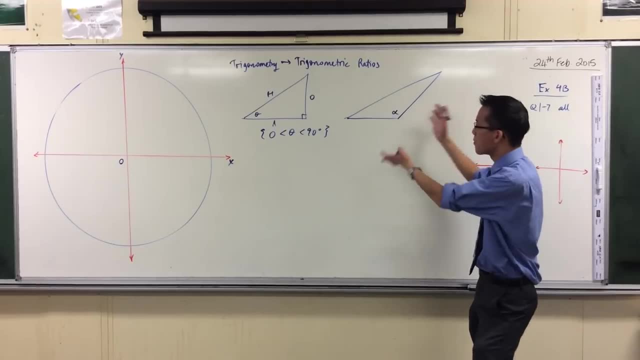 over here. let's call that alpha. can I do trig with that angle, Like if I look at this because it's not acute anymore, right? so here my definitions, my very, very narrow definitions of the trig ratios. they immediately break down right and then 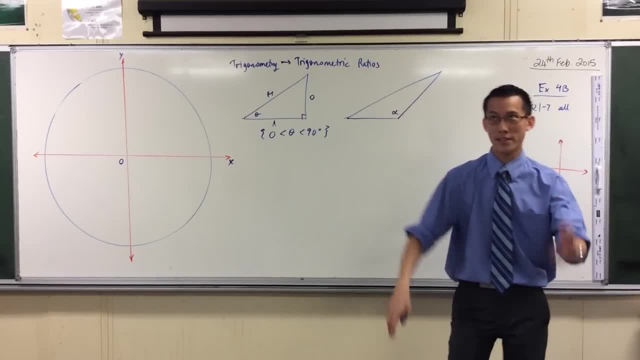 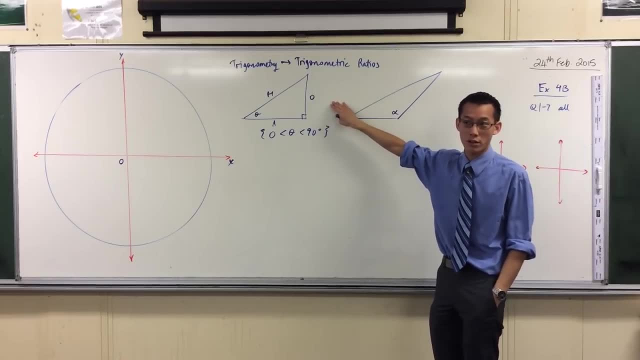 what about trig when the angle's not in a triangle right, where's the opposite? in the hypotenuse there's no hypotenuse. so what do I even do? okay, so this is a nice way to start. right angle triangles are a good beginning. right, because they're. 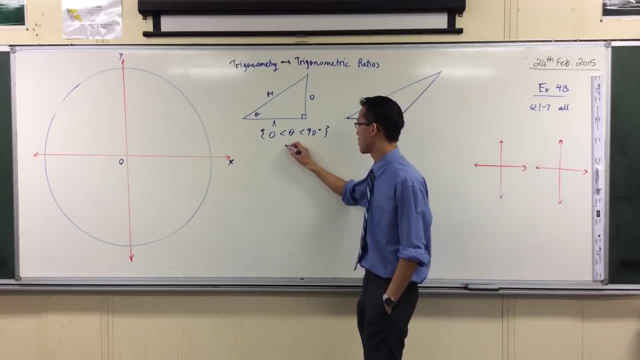 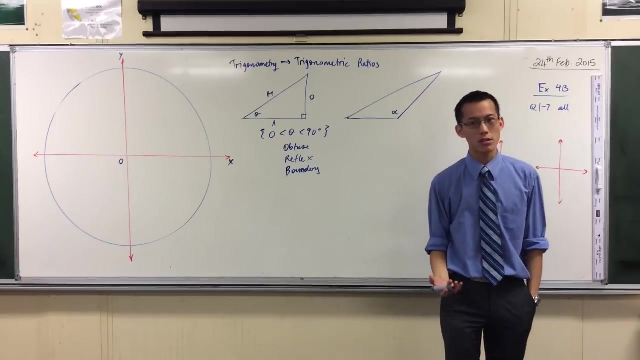 understandable, but um, they're no good right when you think about obtuse angles or reflex angles or bigger angles, or what about just boundary angles? what about 90? right, I have a 90 degree there. what's the sine or cos of tan of 90? how? 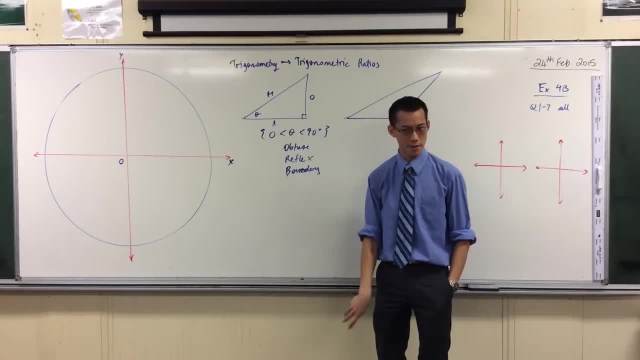 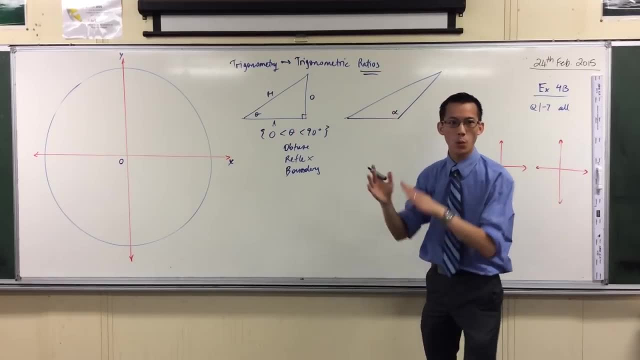 do I work out what these are? this definition isn't gonna fly, okay, and that's why what we're gonna do is we're gonna take this definition and we want to understand not just ratios. we want to move toward trigonometric functions, right. so what we're gonna do is we're gonna take this definition and we want. 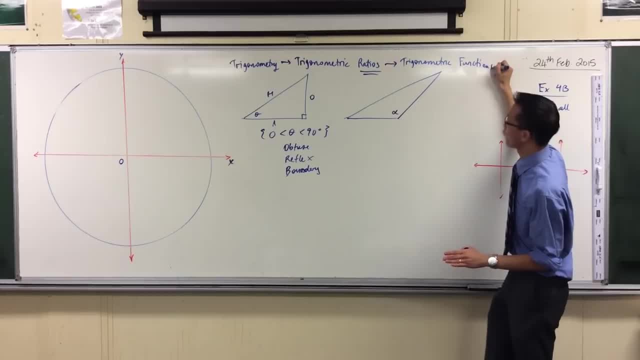 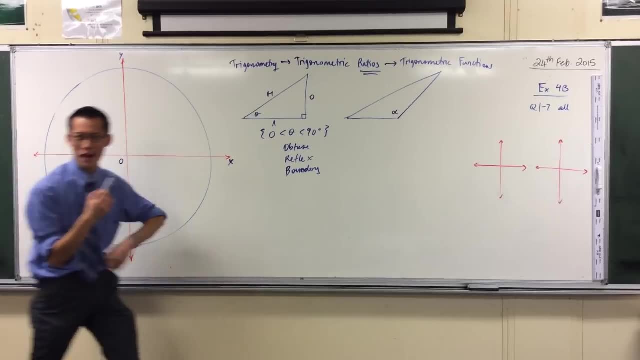 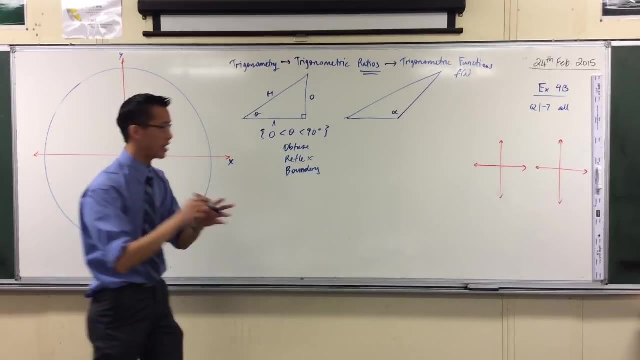 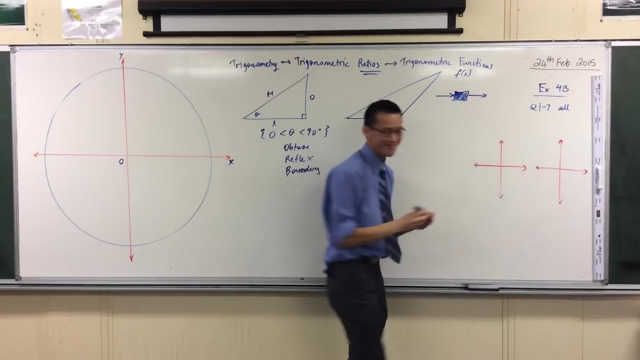 I want you to think back to the first time you heard the word function. right, what is a function? what's a function? we tend to write it with the abbreviation f of X. a function is just something you can stick a number in and get a number out. excuse me, thank you, okay, simple concept. 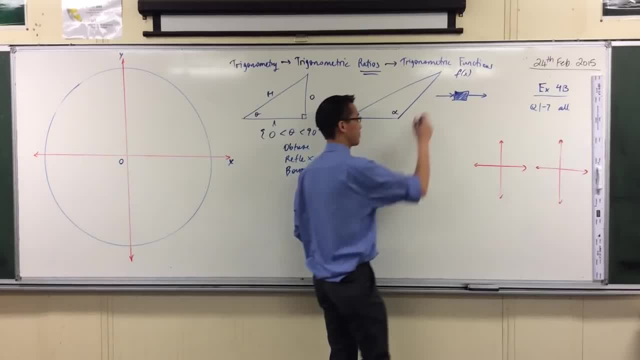 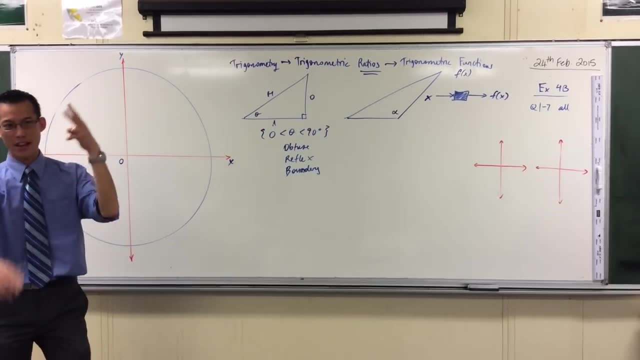 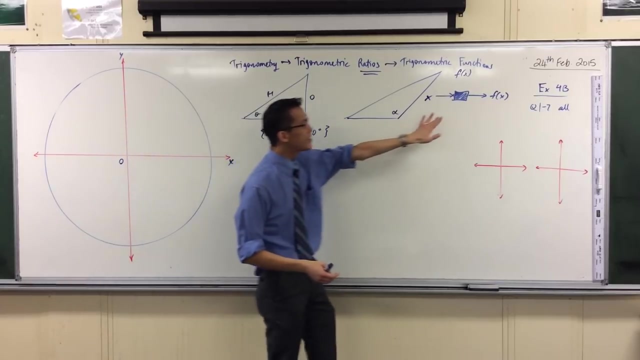 stick a number in, we call it X, and out will come another number. we call that f. right, and we know all kinds of functions already: 2x, 3x minus 1x, squared log of X, blah, blah, blah, blah, blah. okay, so what we want is: can we define sine or cos of tan? 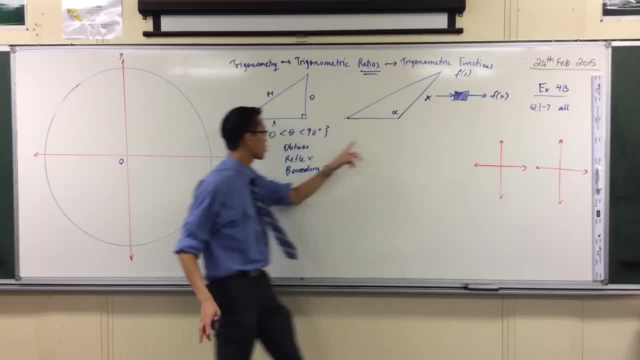 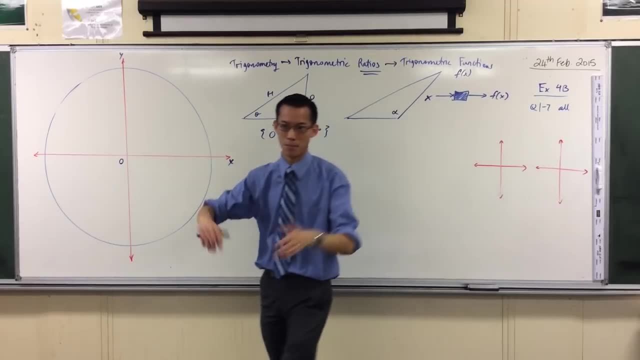 in a way such that I can put any X you like right, not just, not just within this little little spot, such that I can get a value out the other end. I want to. I want to blow open my world and not be stuck in right-angled triangles anymore. 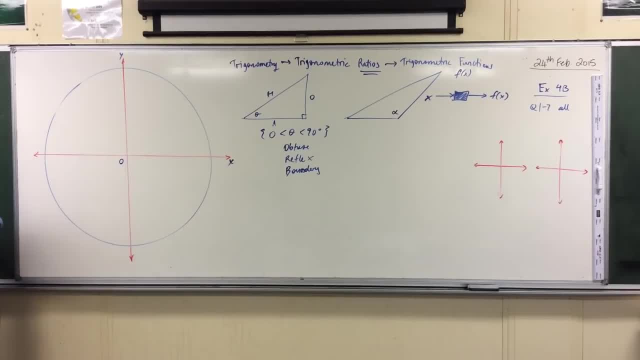 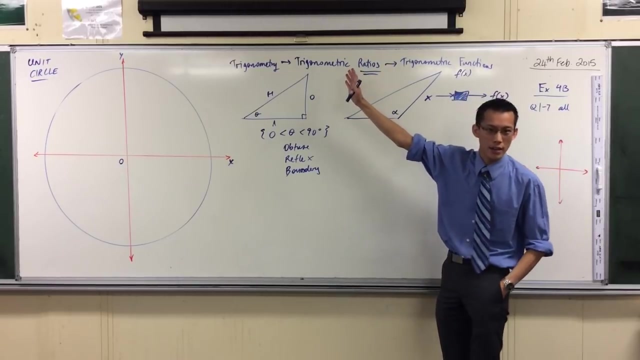 So the way we're going to do this is with a circle, Not just any circle. This is the unit circle, So it has a radius of 1.. There's a radius of 1.. Now, the unit circle is inextricably tied to the trig ratios and the trig functions. 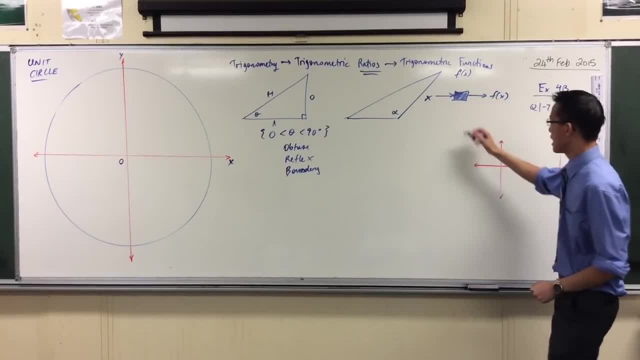 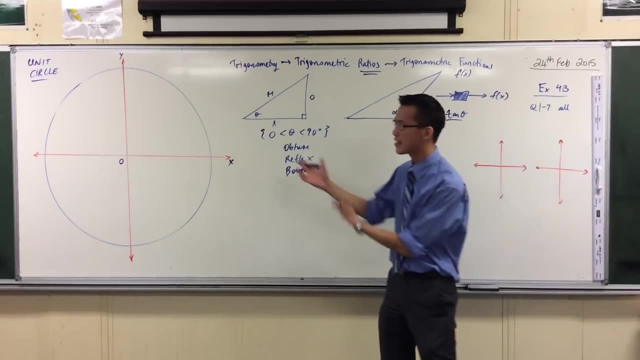 We shouldn't be that surprised because, as we were just explaining, even one of the basic functions, namely tan, is named after a component of a circle, So we should expect that there's some kind of link here. In fact, in some of the older textbooks that you'll have a look at, 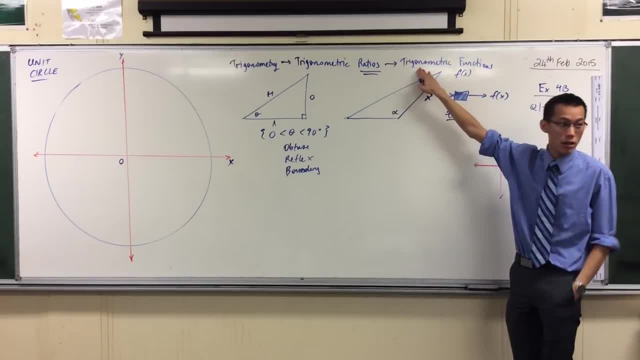 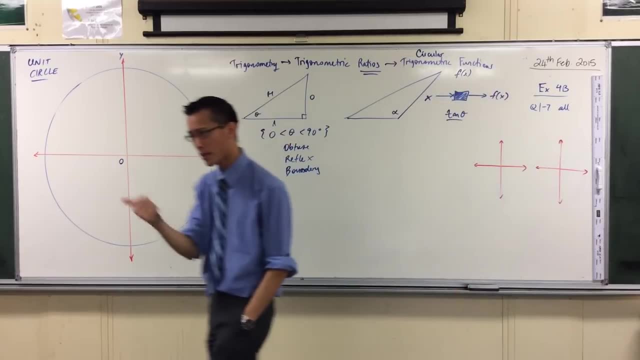 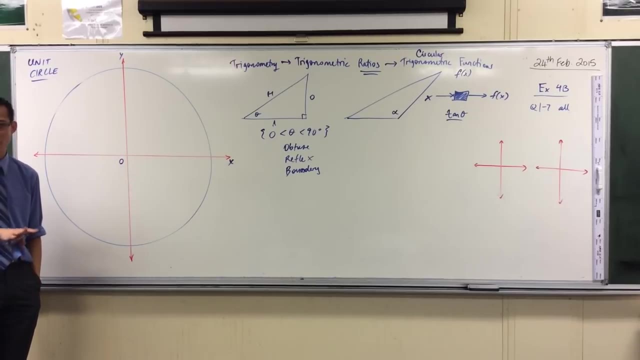 when they're looking at trigonometric functions. the chapter isn't even called trigonometric functions, It's called circular functions- Sine, cos, tan, That's what they're called. So fundamental is the circle to understanding these. So here's the way we're going to go through this. 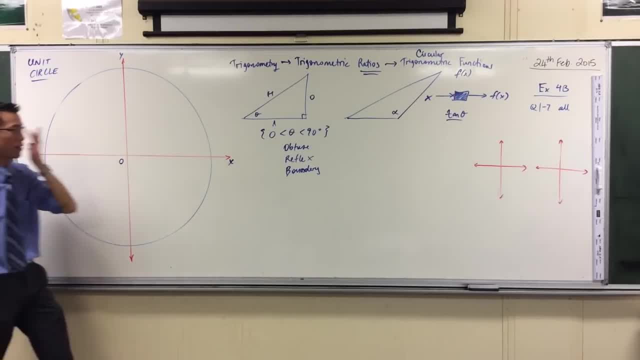 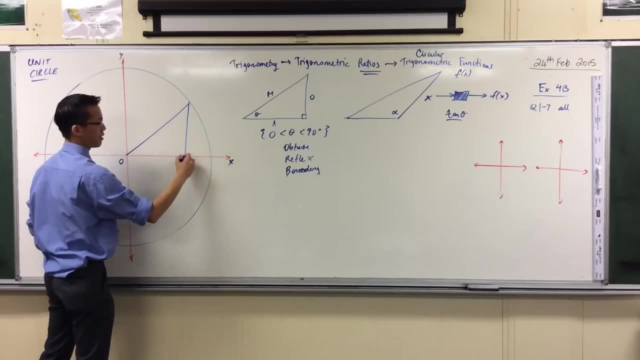 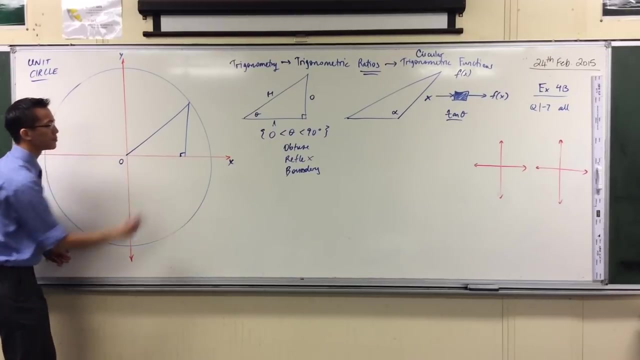 Here's your unit circle, And we're going to put one of these right-angled triangles in our circle, So I'm going to put it right here, in the same orientation as my triangle over here. So there we go. Now I put it here, and so I'm going to put my theta in the same spot as well. 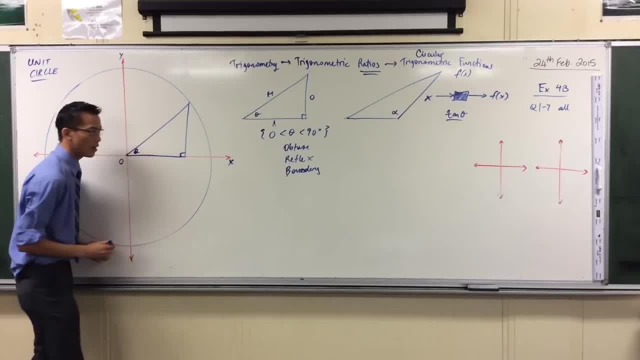 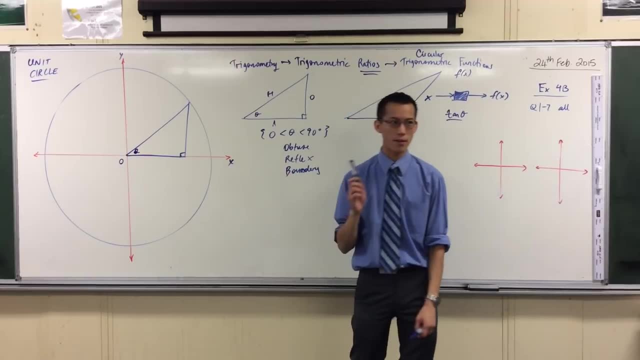 So I actually have a full triangle here. Now, before I go any further, I want to immediately draw your attention to the fact that why do I start here? I start here very on purpose, okay, And it seems a bit confusing. 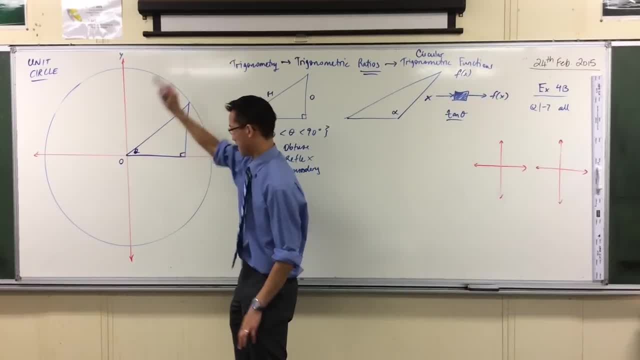 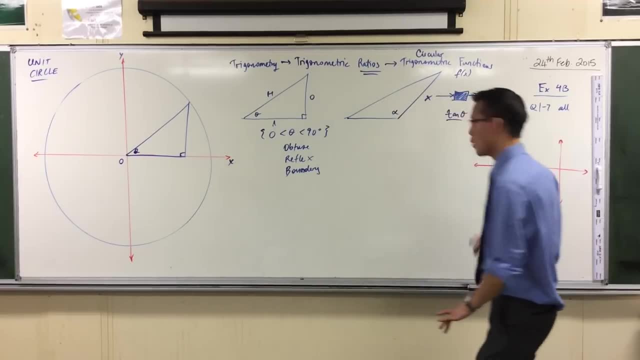 because we have measured angles around a cross-looking thing before when we did bearings. Remember that. Okay, bearings, We've looked at this, But this is a bit weird. Let me show you. When we do bearings, we know how to do north, south, east, west, etc. 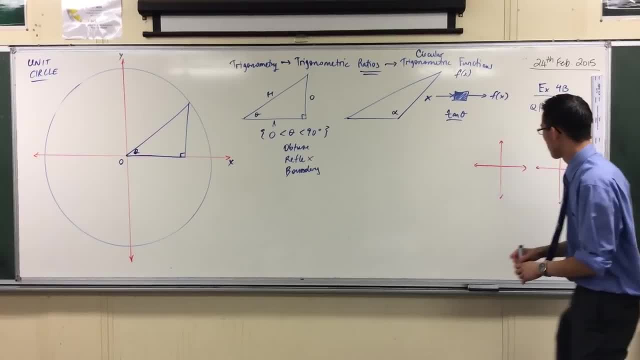 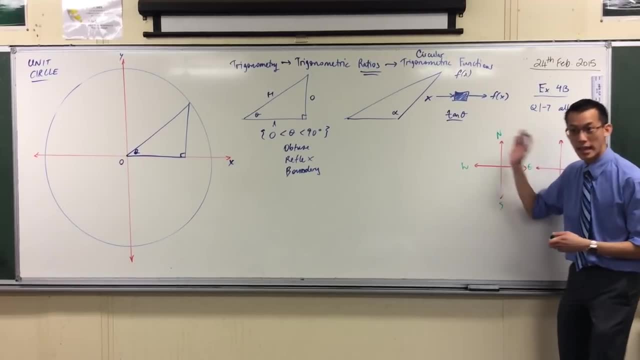 Okay, But true bearings, which I've measured all the way around, where do true bearings begin on a diagram? North east, south west, Where do they begin? Where do they start? They start at north, right, True north, okay. 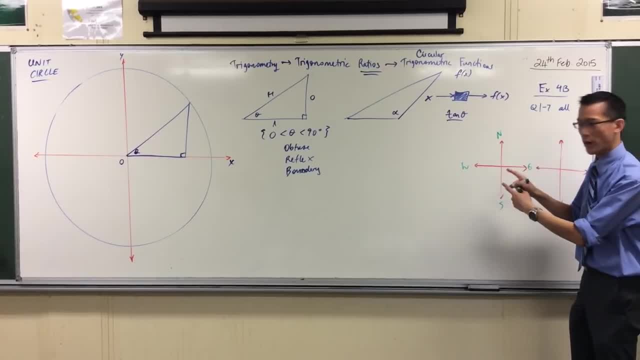 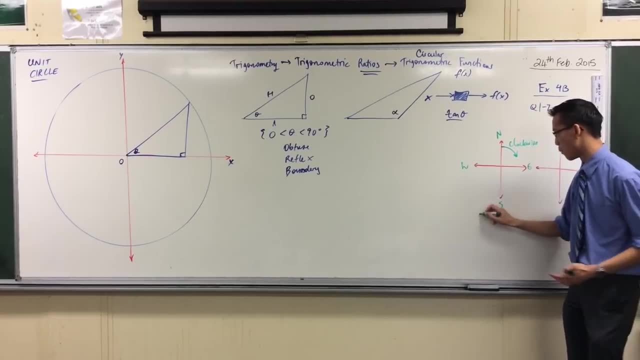 And then we measure in which direction We go. clockwise, okay, And this kind of makes sense, I suppose, for bearings, because north is a sensible place. to begin right, North is like your most important direction. And clockwise, well, it's clockwise because that's the way our clocks go. 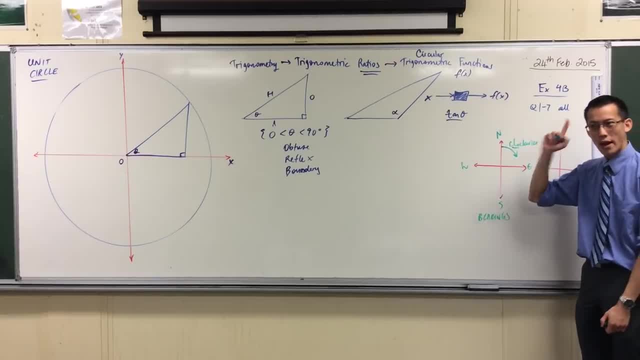 So why not measure that way? Okay, When we're in the unit circle and when we're in trigonometry, okay, things are completely different. So, number one: north is not the starting point, Instead of north being the starting point. 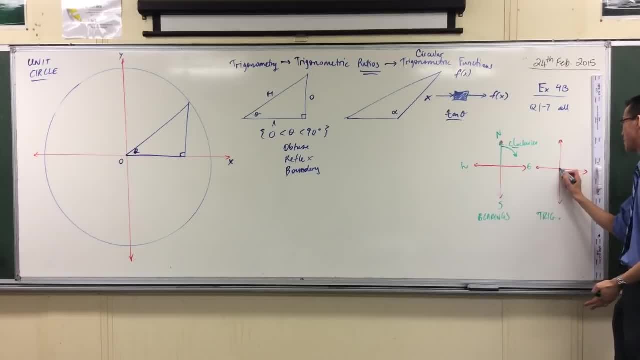 on here. it's well, it's east, It's the x-axis, That's our starting point. Okay, Not only is that different, this is different too. We don't measure clockwise, We measure anticlockwise. Now, just before I give a bit of an explanation, 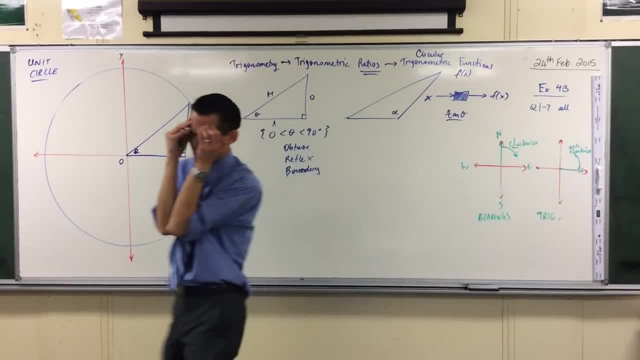 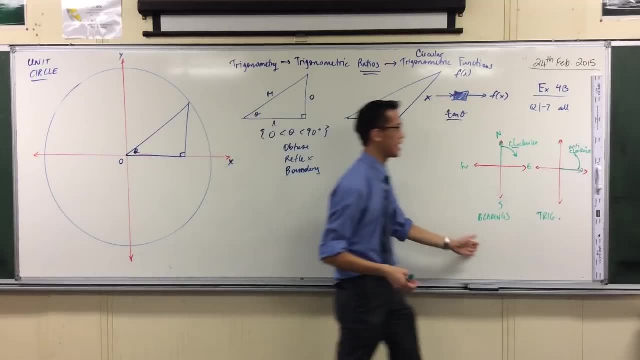 I want you to have a think. Why do they do this right? Why do they make them different? We're both trying to understand the same thing, Angles, okay. Why on earth would they not only change the starting point but the direction? 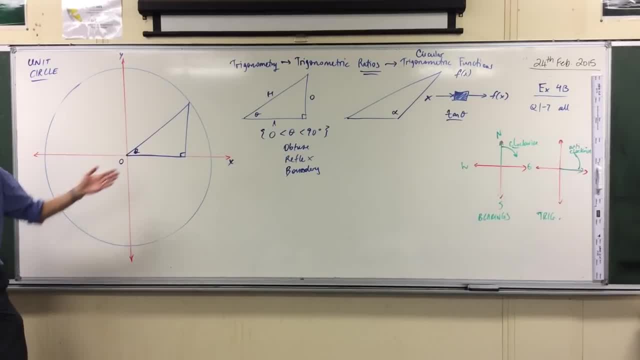 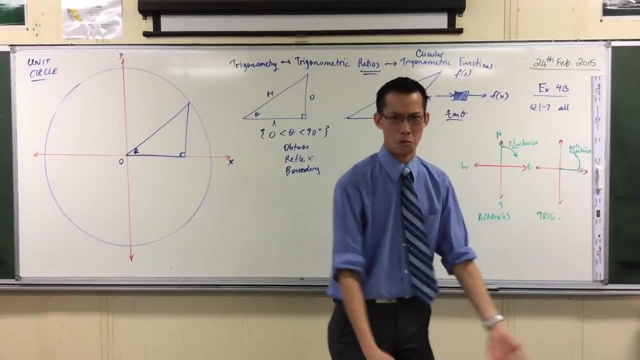 As we go through this, I wonder if you will start to see why this absolutely makes sense in this context. In fact, if anything, the bearings are the ones which are a bit sort of arbitrary. Why start with north? Okay, So that's an important note. 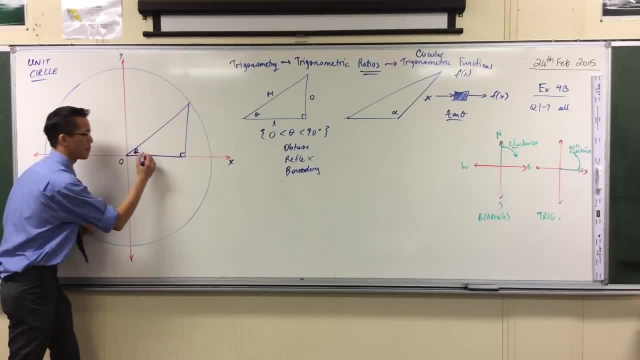 And that's why I'm starting here on the x-axis, and my angle of theta is north, And my angle of theta is measured anticlockwise, You see that? So I'm going around the circle this way. Okay, Now what I want to have a look at is this right angle triangle here. 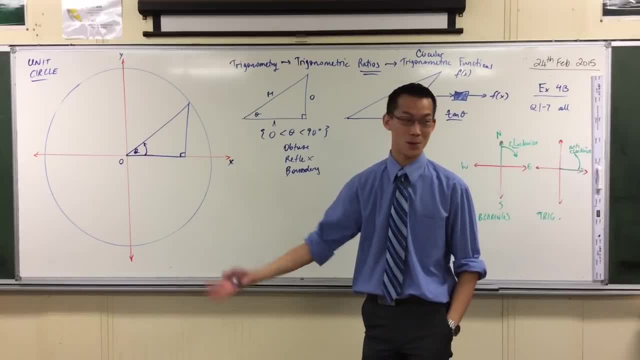 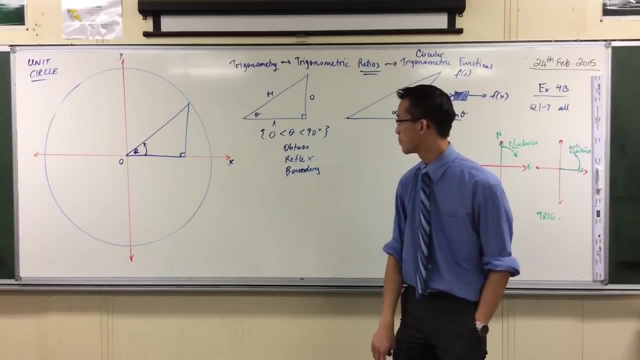 Okay, And just like in our very first question this morning, which is why I started with it right, These sides here I can phrase in terms of the trig ratios: Okay. Now, if I say okay, I've got a point up here. 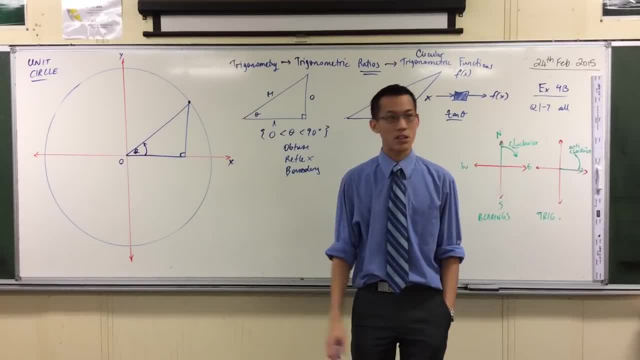 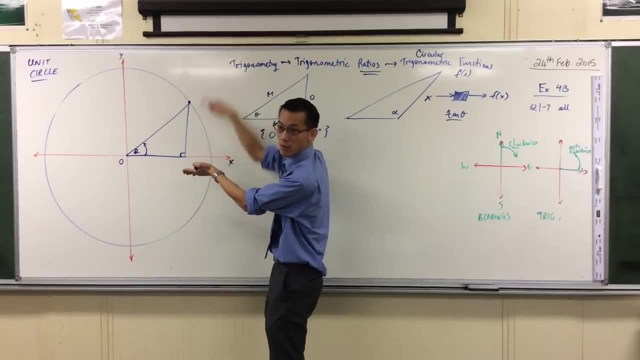 on the circumference of the unit circle. Okay, I want to know what its coordinates are. Its coordinates come from? what's its x-value Horizontal And what's its y-value Vertical? Okay, Don't forget, it's the unit circle. so what's the hypotenuse equal to? 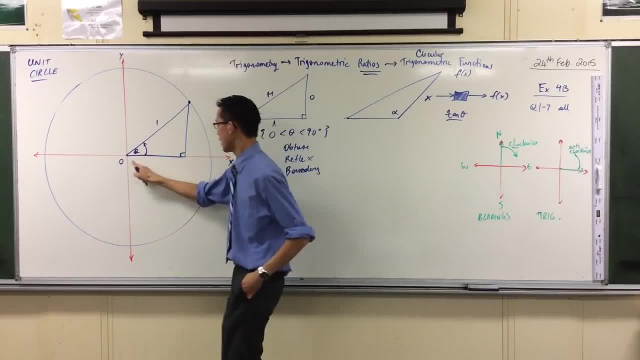 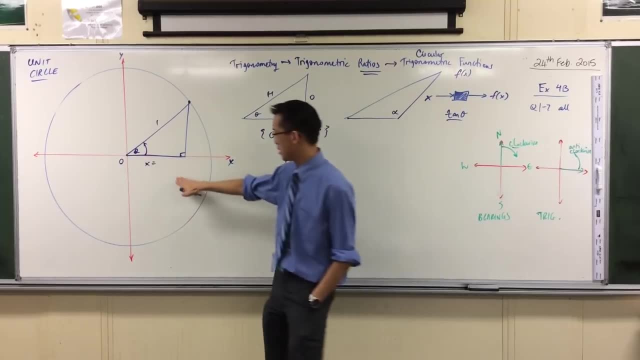 One One, Okay. So down here, here's my x-value. X equals Now, what is x equal to, Right? Well, I've got this side down here and I know what the hypotenuse is. So, being that this is theta, which trig ratio should I choose? 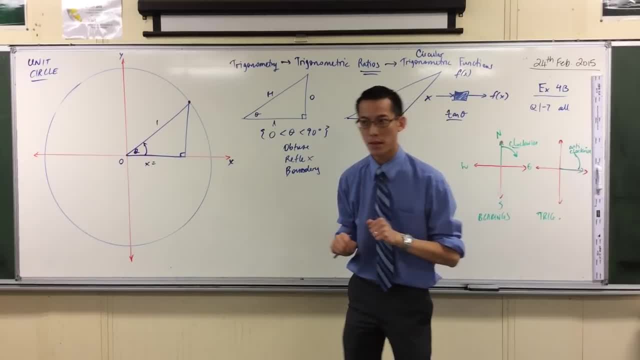 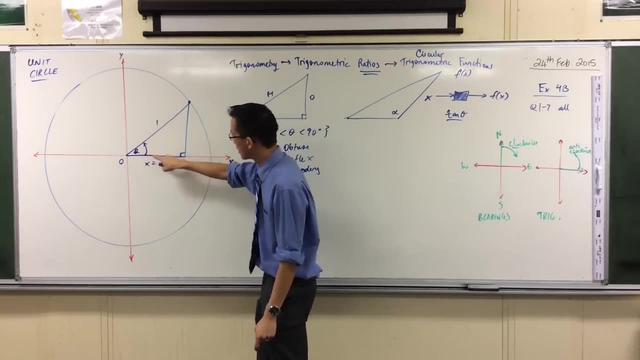 which will relate those two sides. Cos It's cosine, isn't it? Because I've got adjacent and I've got hypotenuse. In fact you can just quickly mentally do it. Cos of theta will be adjacent on hypotenuse. 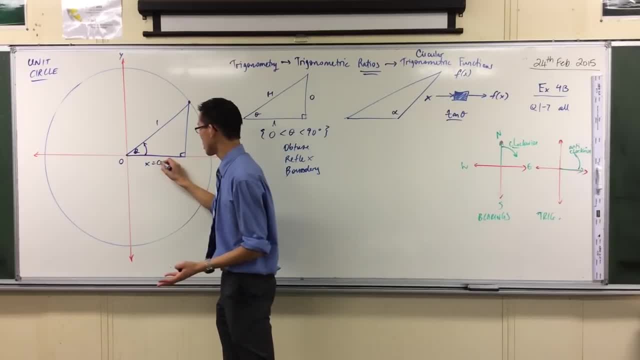 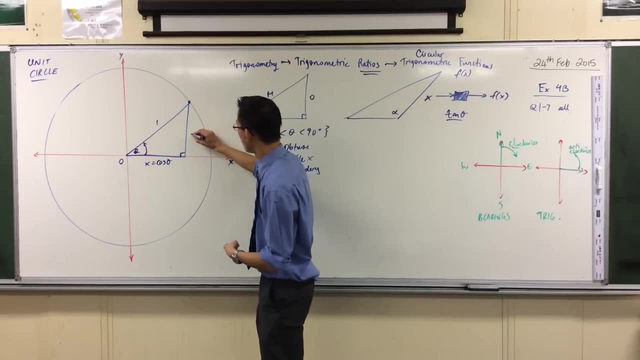 X on one, It's just x, Right. So x is just cos of theta. That's what it's equal to, Okay. In exactly the same way, when I look at y, I've got the opposite side this time, So sine of theta will be opposite. on hypotenuse: 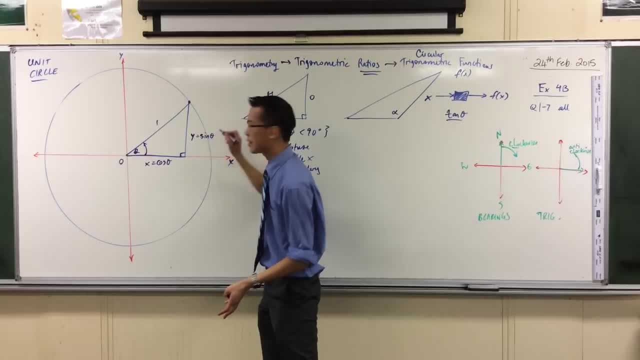 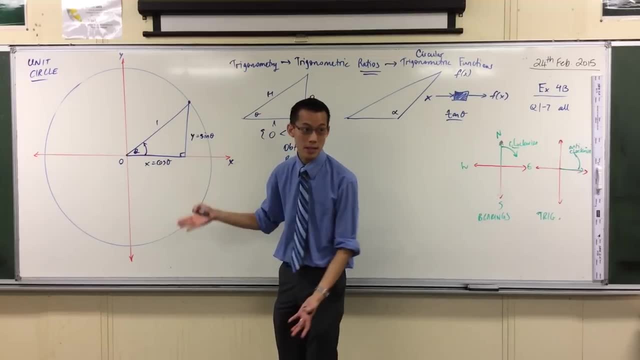 It's just y. So y is equal to sine of theta. Hmm, So now I'm going to stop talking about x and y for a second, because I can just talk in terms of theta, Right? So when I name these coordinates up here, 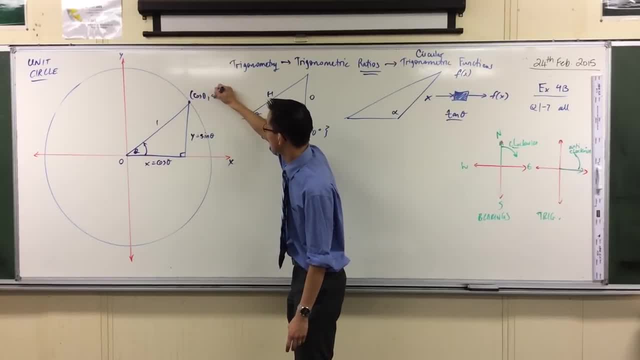 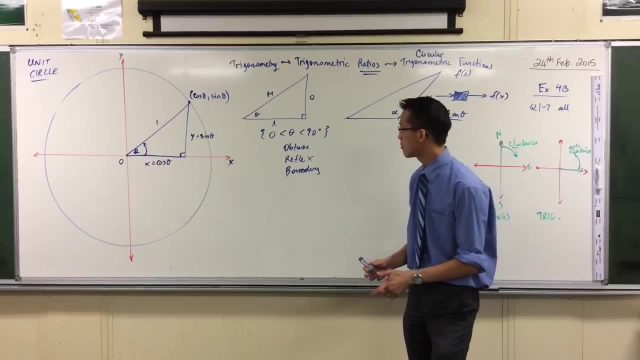 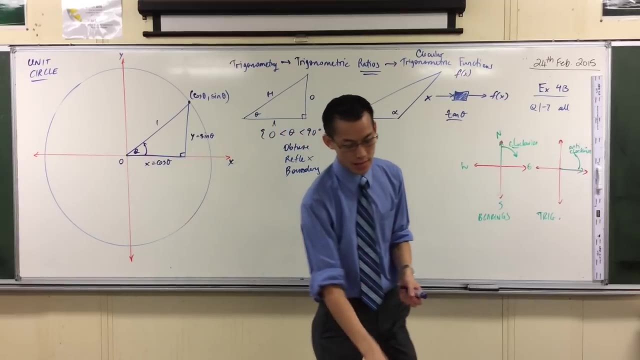 the coordinates of this spot are cos: theta, sine theta, Whatever theta may be. Okay, So what have we done? We have taken this idea here about right angle triangles- right, And we've applied it to the circle, and then we've noted this interesting relationship. 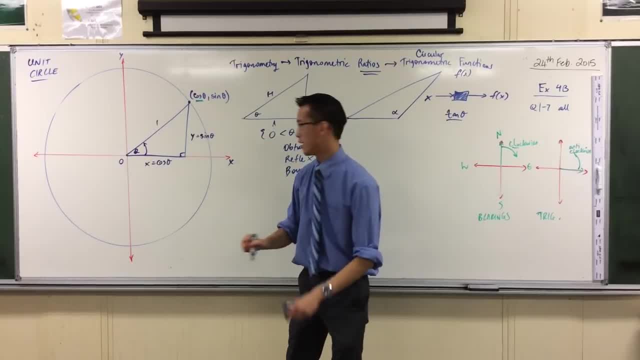 That cos is the x coordinate of the point on the unit circle corresponding to this angle. Let me say that again: The cos theta is the x coordinate of the point on the unit circle that corresponds to that angle Right, And the sine theta is the y value. 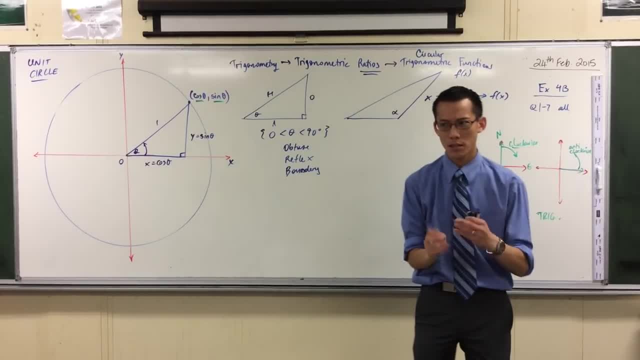 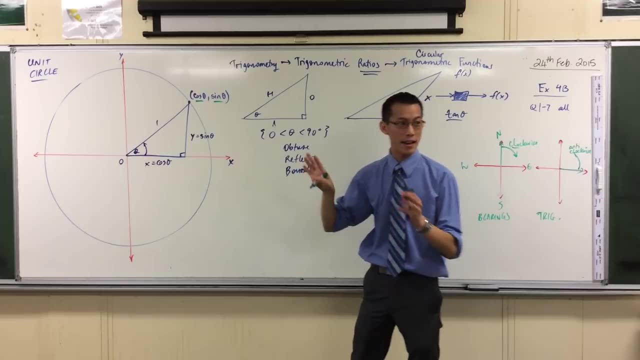 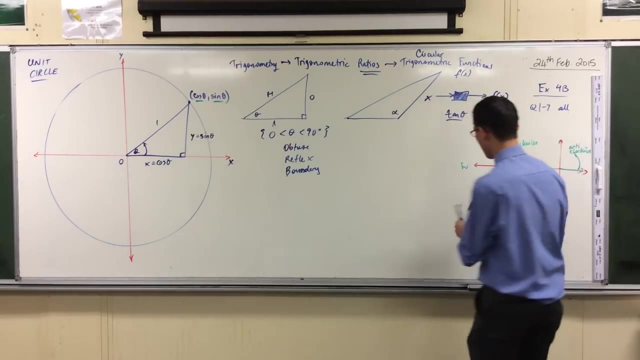 Right, So I'm now going to change gears. This is weird. I am just going to stop defining sine and cos in terms of this triangle. I am now going to define sine and cos in terms of this circle. Okay, Like, in fact, I'll just go over here. 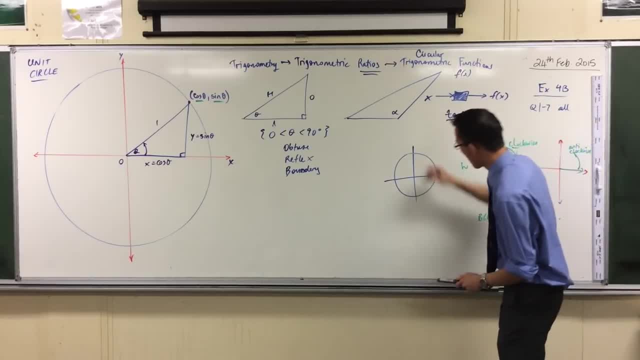 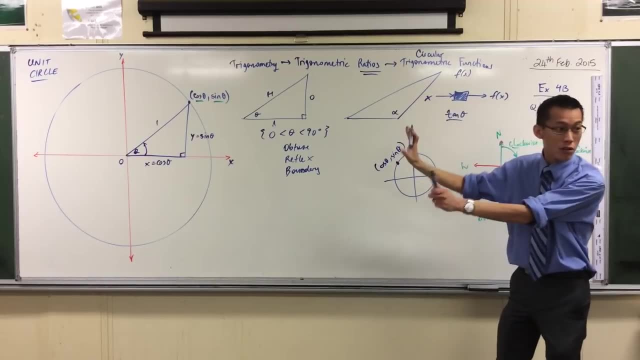 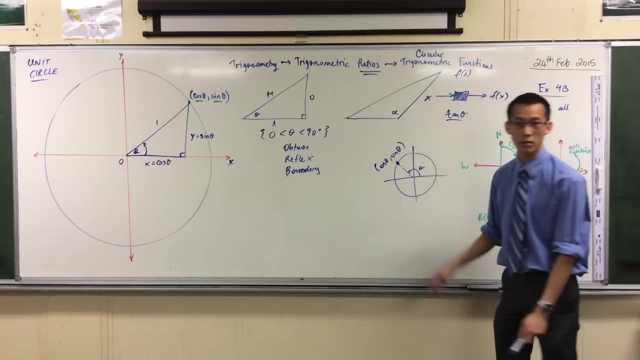 If I drew a new unit circle right And I put like a dot over there, Okay I can define that point as cos theta sine theta, No triangles involved, if measuring this angle around that's theta. Do you see, This is a really big deal.